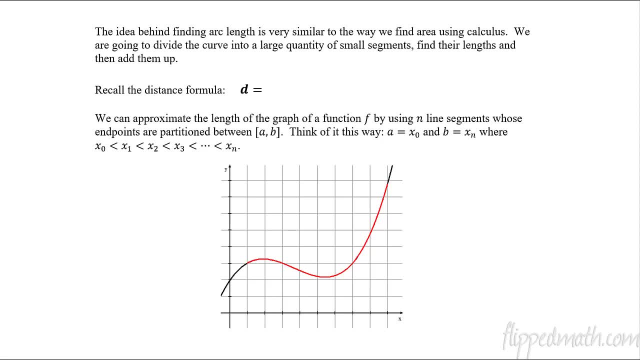 I want to remind you that we've done a lot of things this year already where we take a large quantity of a whole bunch of small little things. So we're going to take a bunch of line segments. and how many line segments are we going to take? When I say a bunch, we're going to make line. 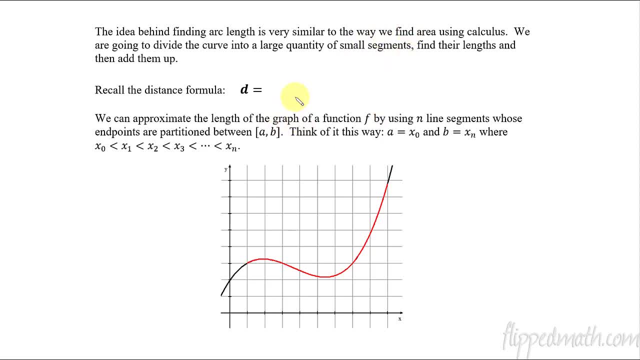 segments approach infinity. So before we get into that, let's remind ourselves what is the distance formula, If you remember, back from geometry days and algebra days, even some pre-algebra days, where really the distance formula is just the Pythagorean theorem. 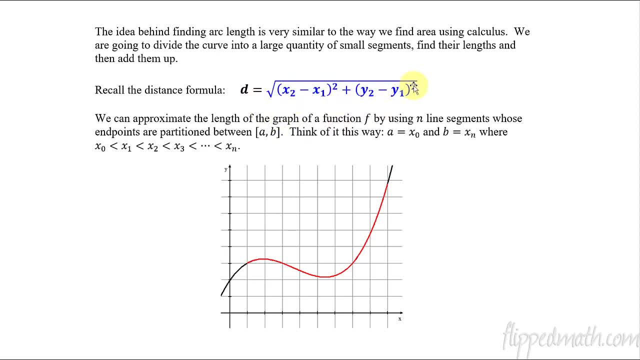 a squared plus b squared, and then you take the square root to find the hypotenuse. That is the distance between two points. So it's the difference in the x's, we add the difference in the y's and so forth. So just get that written down because we will refer to it And then after 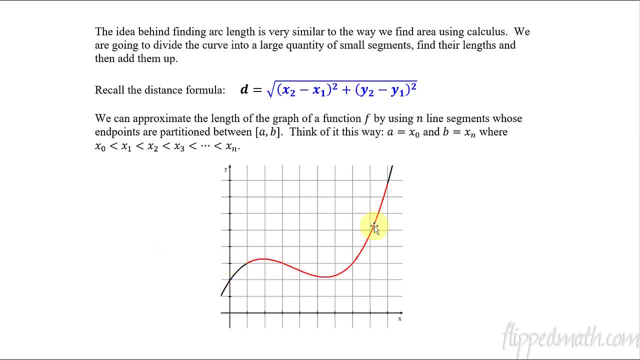 you have that written down. you're going to take the square root of the hypotenuse and you're going to take the square root of the square root, of the square root of the square root. Now we're going to talk about this curve here, So I've highlighted this in red. We're trying to figure out what is. 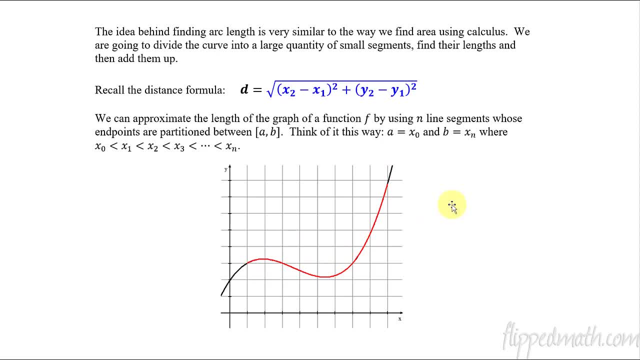 the distance of that thing in red. Well, we can approximate this by taking a bunch of line segments. So I'm going to draw some things that I don't want you to draw, Okay. so again, I do not want you to draw this If I just take a line segment from there to there. let's make that. 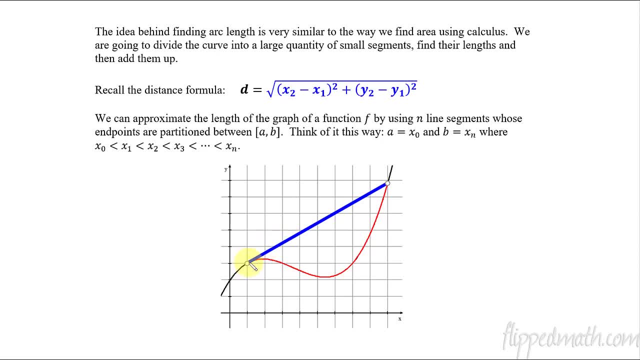 easier to see. There we go. That's better. So here I have a point from the start to the end of the red curved line. This would be an awful approximation if I just drew from one point to the other. It would be an awful approximation if I just drew from one point to the other. It would. 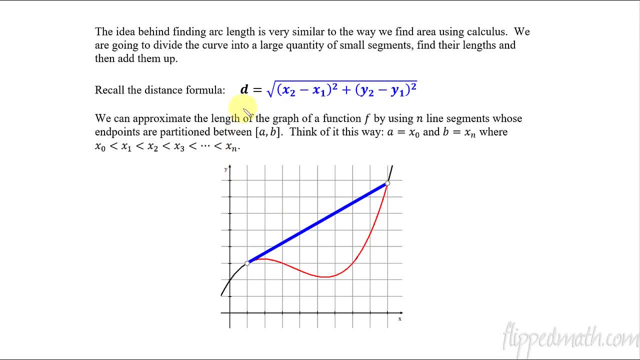 is an approximation, just not very good. But I could find that distance by doing the Pythagorean theorem right. I could take here the change in x, this direction, and then go up and find the change in y. So it would be the change in x. I'll say delta x and then delta y and then do the square. 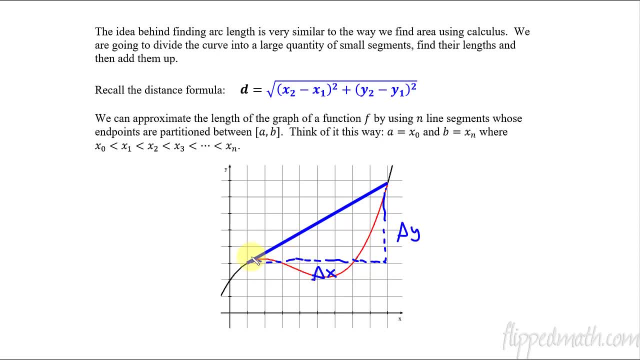 plus square, take the square root of the sum of those things, and then you have that distance right, That's the distance formula. But again, we're not writing this down. I just want to show you a couple little things. I'll tell you when to start writing. So here's another example. 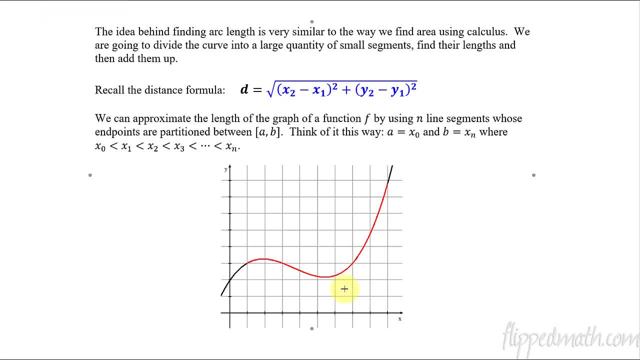 What if I, instead of having one line segment, what if I had two line segments? So from the beginning point to the middle, and then again if I did from the middle to the end, So now I would have two line segments. This is still an approximation of the red curve. If I found the 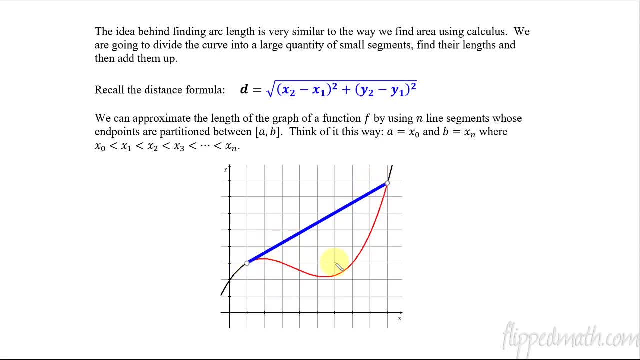 So here I have a point from the start to the end of the red curved line. This would be an awful approximation If I just drew from one point to the other. it would be an awful approximation. It is an approximation just not very good. But I could find that distance by doing the Pythagorean. 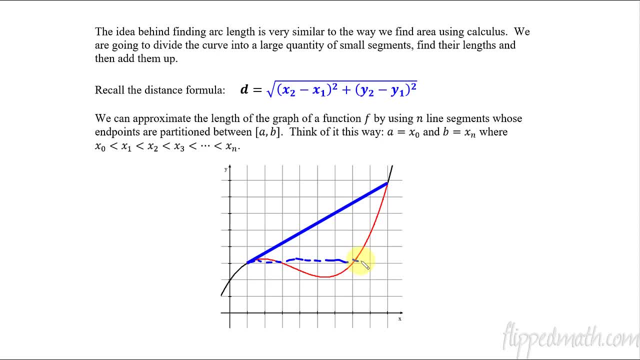 theorem right, I could take here the change in x, this direction, and then go up and find the change in y, So it would be the change in x. I'll say delta x and then delta y, and then do the square plus square. Take the square root of the sum of those things and then you have that distance. 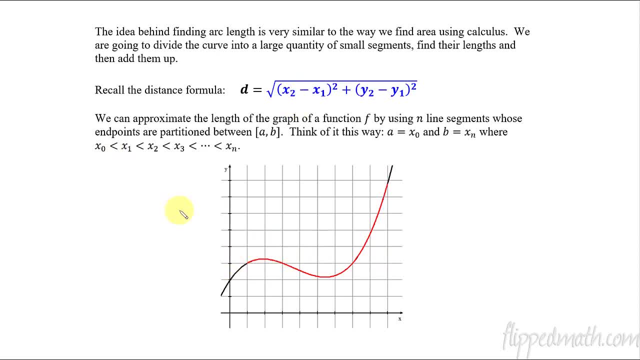 right, That's the distance formula. But again, we're not writing this down. I just want to show you a couple little things. I'll tell you when to start writing. So here's another example: What if I, instead of having one line segment, what if I had two line segments? So, from the 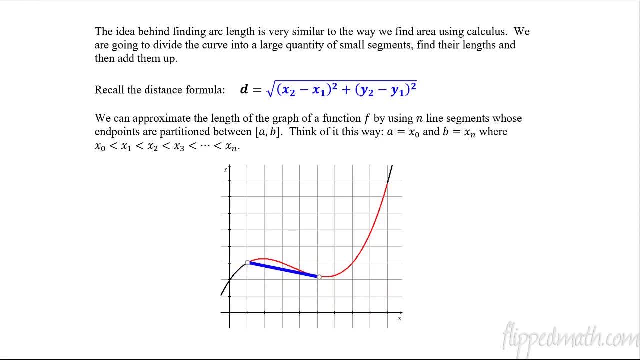 beginning point to the middle, and then again, if I did, from the middle to the end, So now I would have two line segments. This is still an approximation of the red curve. If I found the distance of those two line segments, it still is not a very good approximation. 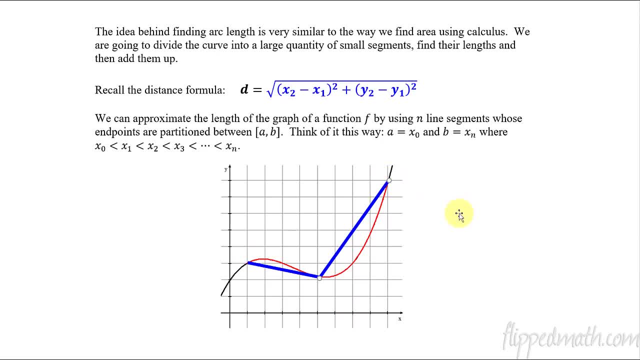 but it's definitely better than the one I had where it was just one line segment right. And what would I do to find these lengths? It would be the same thing as just taking the Pythagorean theorem, the distance formula, like what we have up here. 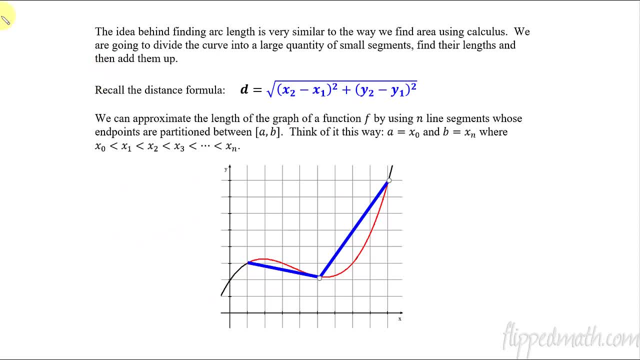 Okay, So now this is the one I want you to write down. Okay, So let me erase this and you write down the following: This time we're going to do four line segments, So we're going to start here and go there, and then I'll go from that point to that point. 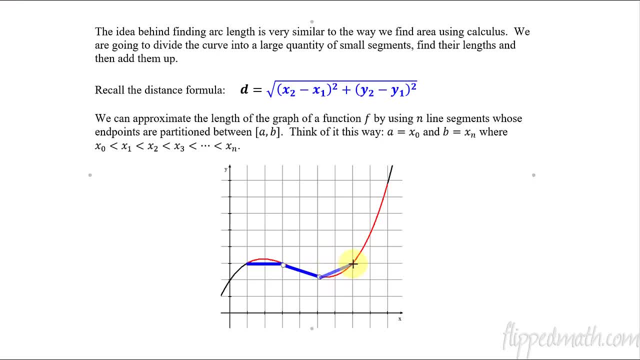 So the four line segments means these are two x values in length, right, Yeah, Two x values in a length each, so that one and then up to here, so you can see if I have more and more line segments on a given interval. the more line segments I have, the better approximation the length of those line. 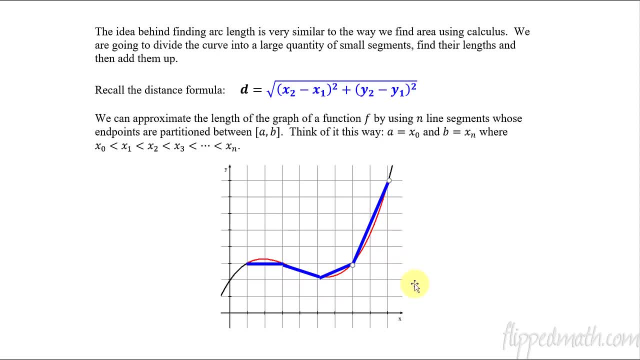 segments will be to the arc length. so this is where the calculus comes in, because we would have the number of segments approach infinity. so we're going to label this. let me get my pin: this is a, this here is b. so we're going from a to b on an interval and our first a is the initial x. 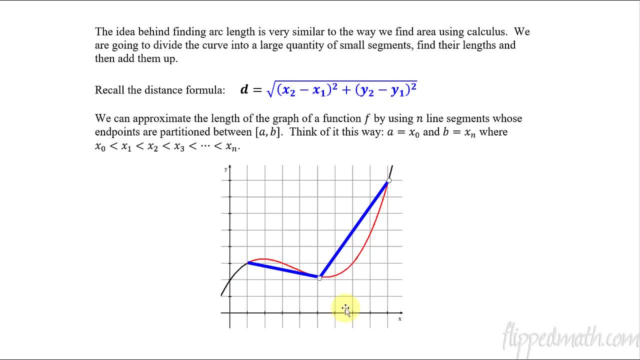 distance of those two line segments. it still is not a very good approximation, but it's definitely better than the one I had where it was just one line segment right. And what would I do to find these lengths? It would be the same thing as just taking the Pythagorean theorem, the distance 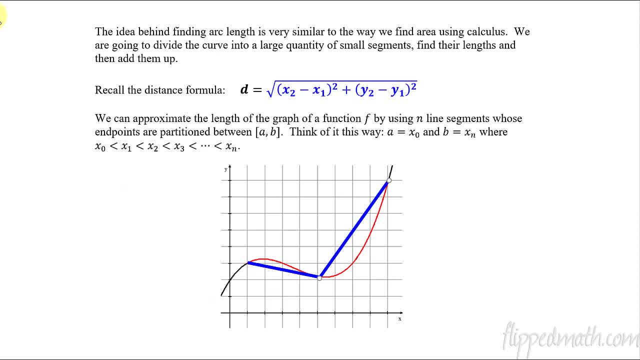 formula like what we have up here. Okay, so now this is the one I want you to write down. Okay, let me erase this- and you write down the following: This time we're going to do four line segments, So we're going to start here and go there, and then I'll go from that point to 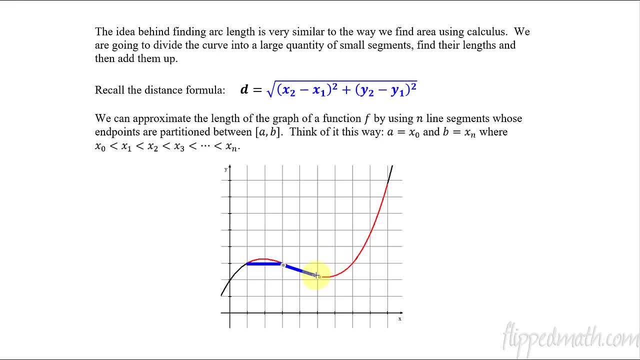 that point. So the four line segments means these are two x values in length, right Yeah, Two x values in length each, so that one, and then up to here. So you can see if I have more and more line segments on a given interval. the more line segments I have, the better approximation. 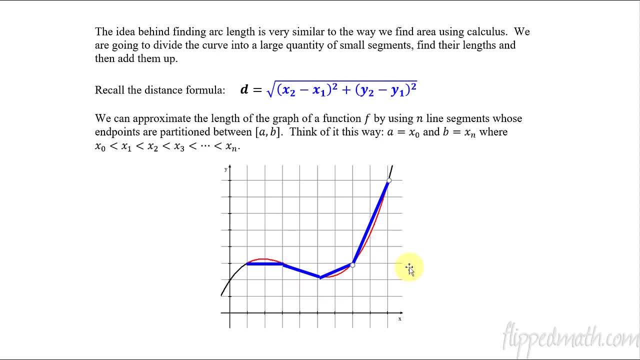 the length of those line segments will be to the arc length. So this is where the calculus comes in, because we would have the number of segments approach infinity. So we're going to label this- Let me get my pen- This is a, this here is b. So we're going from a to b. 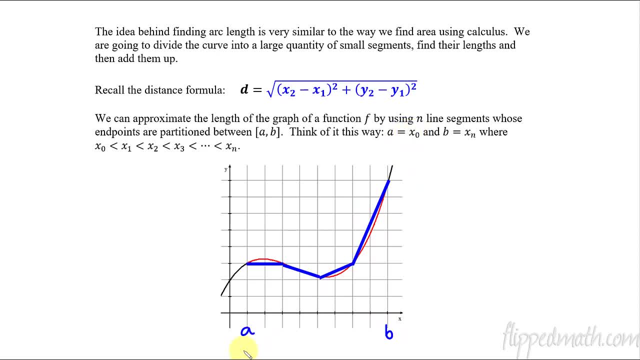 on an interval and our first a is the initial x and our last b that would be the x value of n, representing the nth line segment. because this here would be our x to the 1,, this here would be our x to the 2,, this here would be our x to the 3, and then this would: 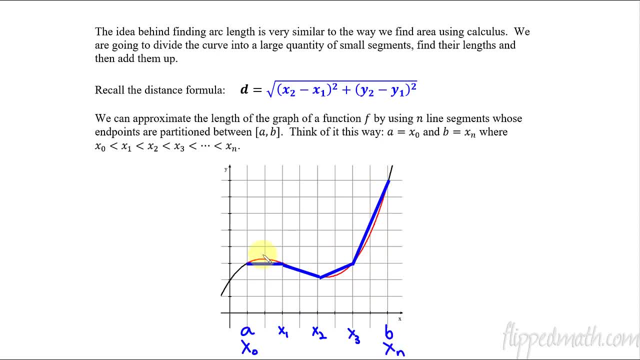 be our x to the 4, representing the fourth line segment, And then we just find the length of each of those little segments by using the distance formula. So what's crazy is that this leads us to the formula that I'm going to show you here Now. the proof of this I'm going to put. 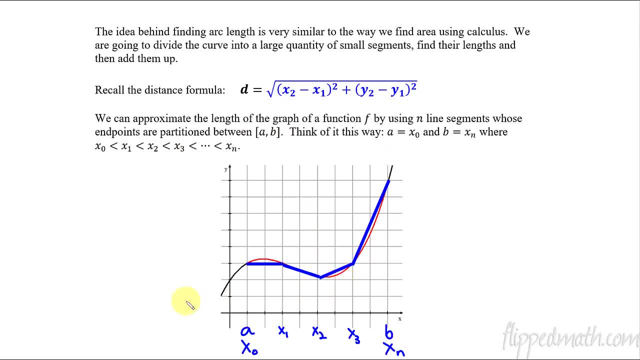 the proof at the very end of the video lesson. The proof actually. you don't have to understand exactly how to do the whole proof of it. I'm going to show it to you because it is a good mathematical understanding to know how we derive this equation here for arc length. But they're 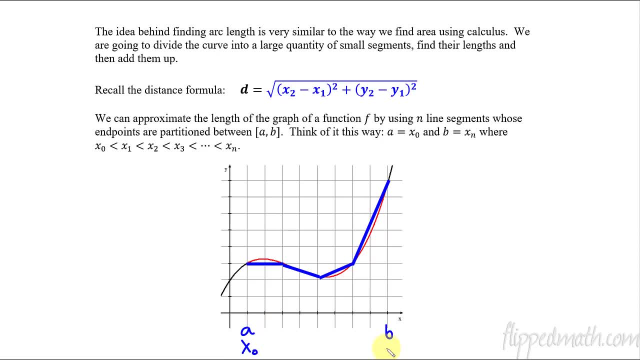 and our last b, that would be the x value of n, representing the nth line segment, because this here would be our x to the one, this here would be our x to the two, this here would be our x to the three, and then this would be our x to the four, representing the fourth line segment. 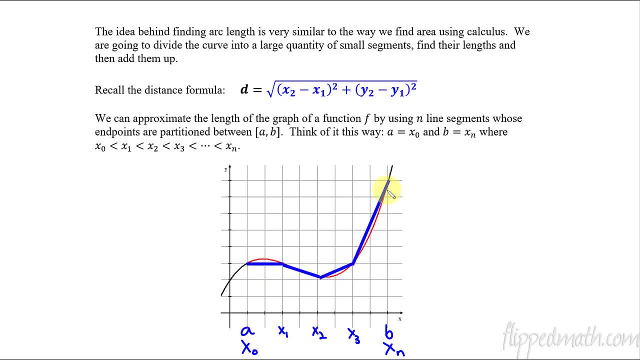 and then we just find the length of each of those little segments by using the distance formula. so what's crazy is that this leads us to the formula that I'm going to show you here now, the proof of this. I'm going to put the proof at the very end of the video lesson. the proof actually. 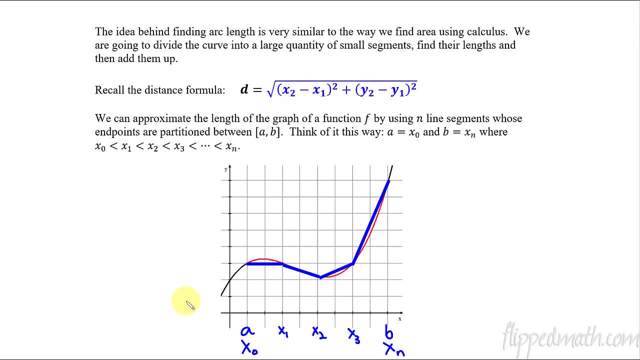 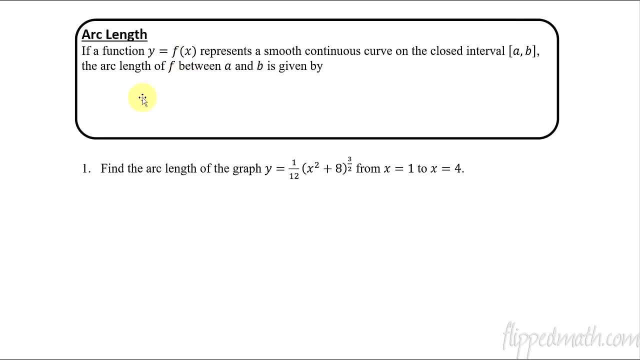 you don't have to understand exactly how to do the whole proof of it. I'm going to show it to you because it is a good mathematical understanding to know how we derive this, this equation here for arc length. but they're not going to test that on the AP exam. they will test your ability to use. 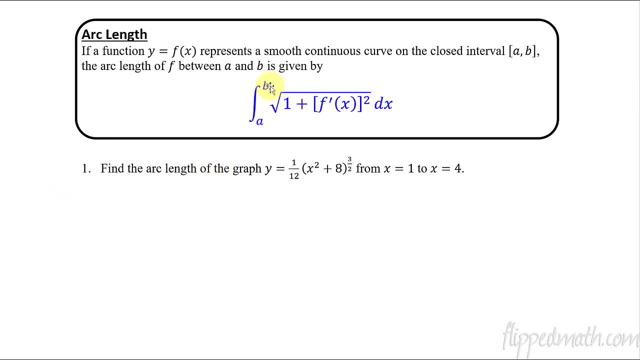 this. so we're going to have an integral from a to b and then the square root. the square root does come from the distance formula: square root of one plus f prime squared. this is weird. where does this all come from? I'll show you that in our proof at the end. but you could think of f prime. I like to think. 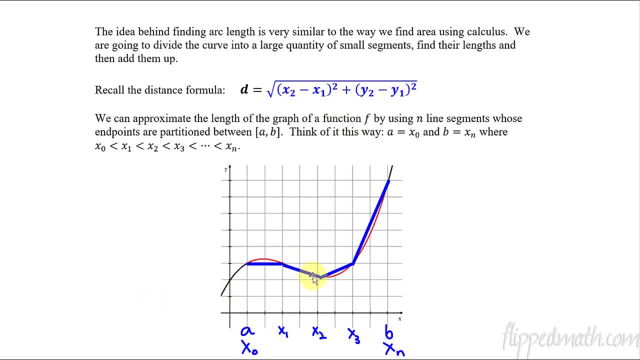 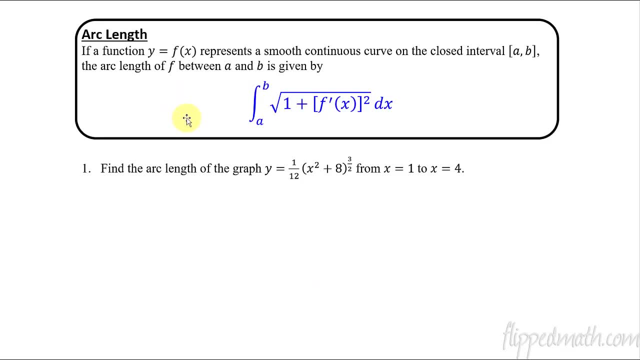 of it a little bit as these little, all these line segments. the more line segments you get, the closer and closer they're going to actually approach a tangent line, a tiny little tangent line which would be f prime. that's kind of how it works. so we're going to have an integral from a to b and 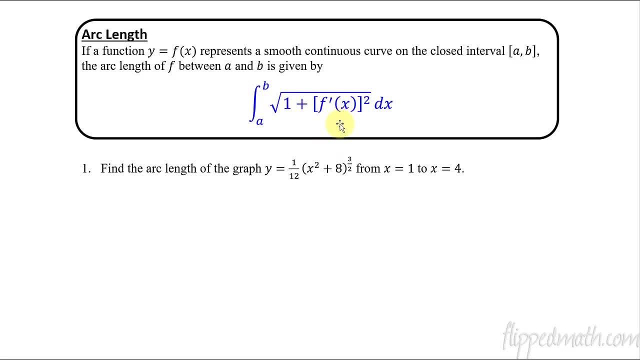 what helps me remember it, but it's one plus f prime squared. common mistake here: that when kids start using this, they only do f squared and not f prime squared, so just be careful about that, all right. so let's learn how to set this up and how we would solve these. we're going to find the 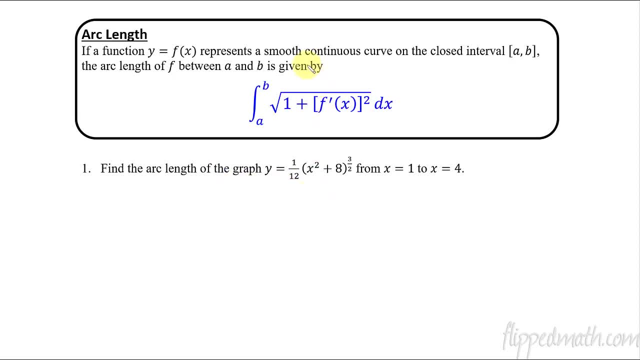 arc length of this graph. oh wait, I should have mentioned this. it needs to be a smooth, continuous curve. so if our curve is not nice and smooth, if it had a corner in it, then this does not work to find the arc length, or if it's discontinuous, then it wouldn't work. so in other words, it needs to be. 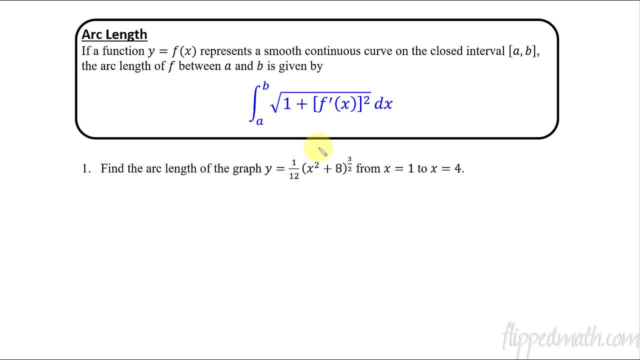 a nice con, differentiable function, continuous and smooth the whole way, in order for us to find the arc length. all right, let's do this one now. before we can set up the, the integral for the arc length, we need to know f prime. so let's, that's always something to remember right away. we're 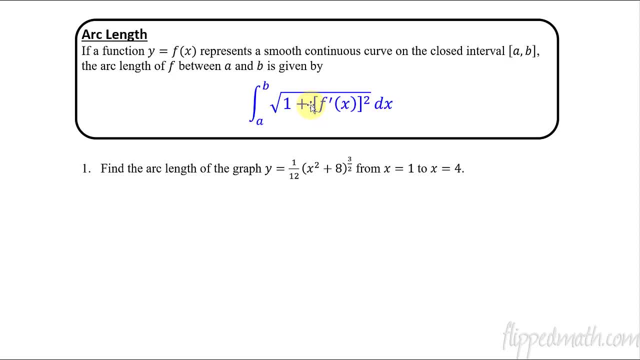 not going to test that on the AP exam. They will test your ability to use this. So we're going to have an integral from a to b and then the square root. the square root does come from the distance formula: square root of one plus f, prime squared. this is weird. where does this all come from? i'll 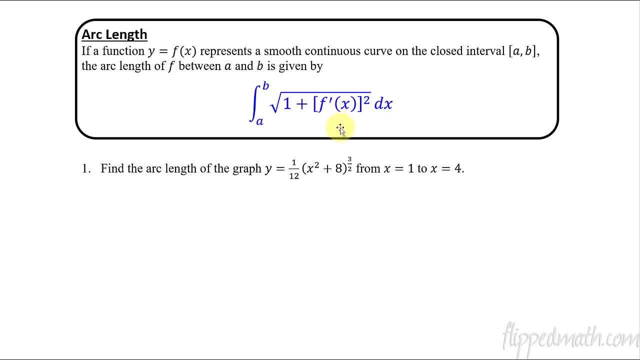 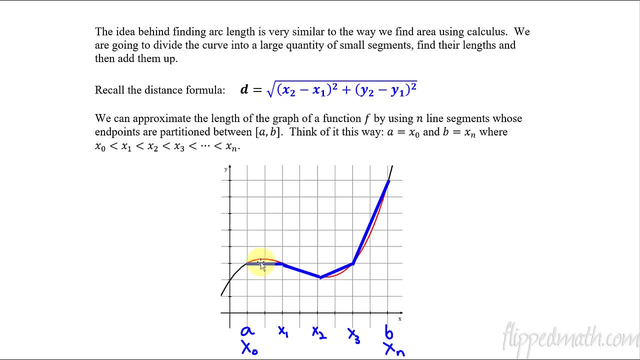 show you that in our proof at the end. but you could think of f prime. i like to think of it a little bit as these little, all these line segments. the more line segments you get, the closer and closer they're going to actually approach a tangent line, a tiny little tangent line which 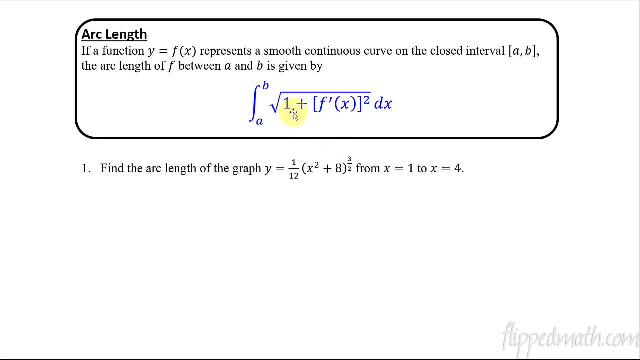 would be f prime. that's kind of how what helps me remember it, but it's one plus f prime squared. common mistake here: that when kids start using this, they only do f squared and not f prime squared, so just be careful about that, all right. so let's learn how to set this up and how we would. 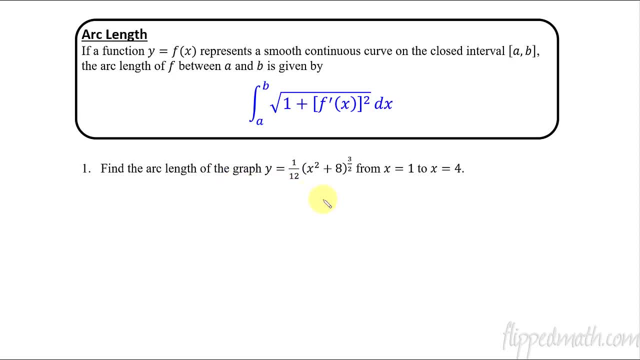 solve these. we're going to find the arc length of this graph. oh wait, i should have mentioned this. it needs to be a smooth, continuous curve. so if our curve is not nice and smooth, if it had a corner in it, then this does not work to find the arc length, or if it's discontinuous, then it would. 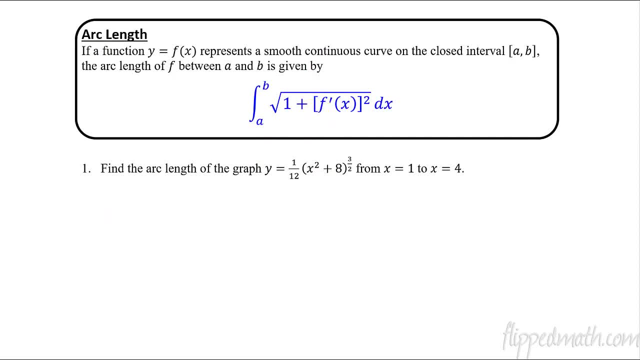 work. So in other words, it needs to be a nice, differentiable function, continuous and smooth the whole way in order for us to find the arc length. All right, let's do this one Now. before we can set up the integral for the arc length, we need to know f prime. So that's always something. 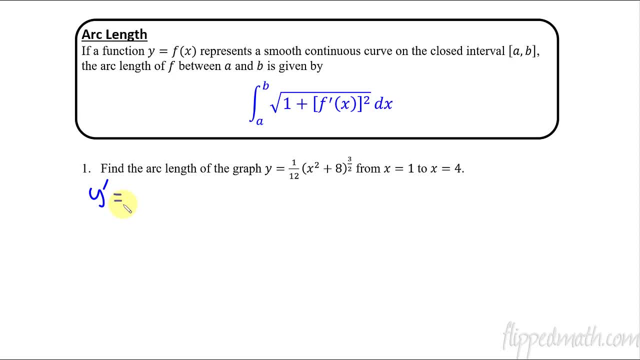 to remember right away. We're going to have to figure out what does y prime equals. So the three halves comes down, three halves times the 1, 12th, and then we have the inside left alone. so x squared plus eight, and then now the three halves subtract one. it's now a one half, and then times. 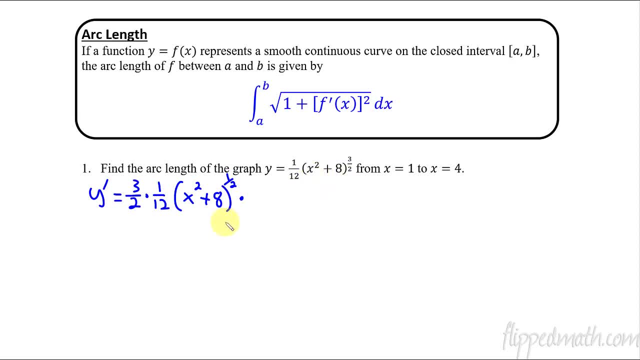 it by the chain rule. derivative of the inside of this is just going to be two x. Okay, so now we can clean up just the derivative here, So that two there is going to cancel with that two, and then this three and the 12 is going to reduce to one fourth. All right, good, that makes this a lot. 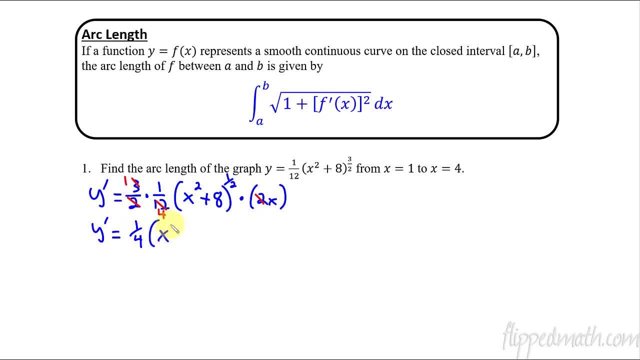 cleaner. So I have one fourth and then x squared plus eight raised to the one half, or in other words the square root of x squared plus eight. Oh man, I'm glad I just caught this before I move on. Hold on, let's change that one. I forgot this. 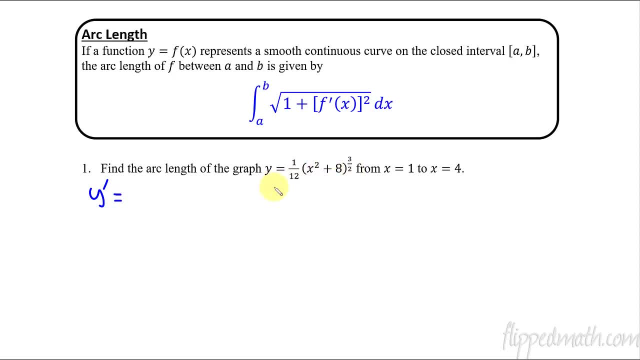 going to have to figure out. what does y prime equals? so the three halves comes down, three halves times the 1, 12th, and then we have the inside left alone. so x squared plus 8, and then now the three halves subtraction one, it's now a 1 half, and then times it by the chain rule derivative of the inside of this is: 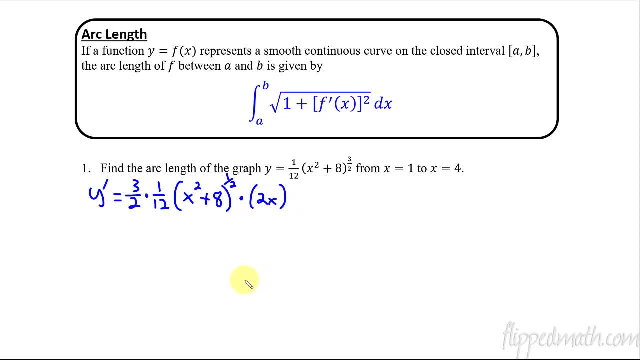 just going to be 2x. okay, so now we can clean up just the derivative here, so that 2 there is going to cancel with that 2, and then this 3 and the 12 is going to reduce to 1, 4th. all right, good that. 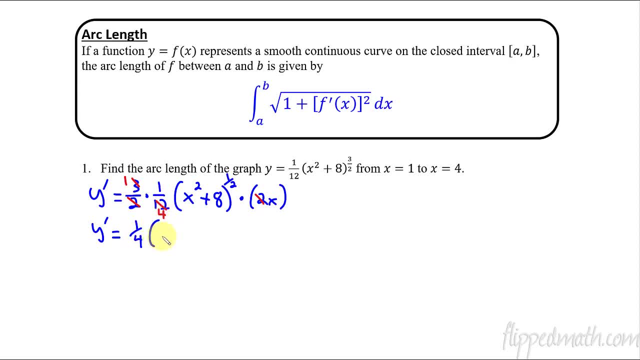 makes this a lot cleaner. so I have 1 4th and then x squared plus 8 raised to the 1 half, or in other words the square root of x squared plus 8 raised to the 1 half. so that's going to be 1 half, and then 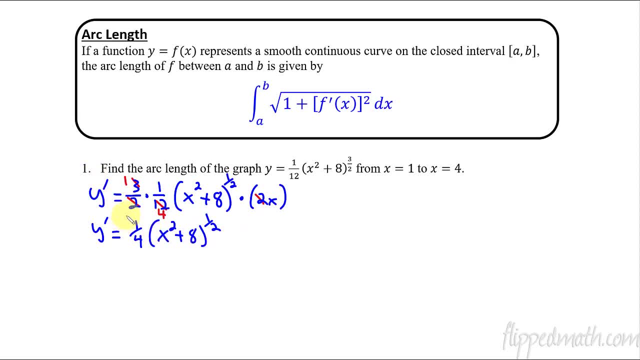 x squared plus 8. oh man, I'm glad I just caught this before I move on. hold on, let's change that. one forgot this X right there. that X is supposed to be there, so X over 4. yeah, that's important. okay, so now I'm going to set up my integral. that represents the arc length, so let's go integral. 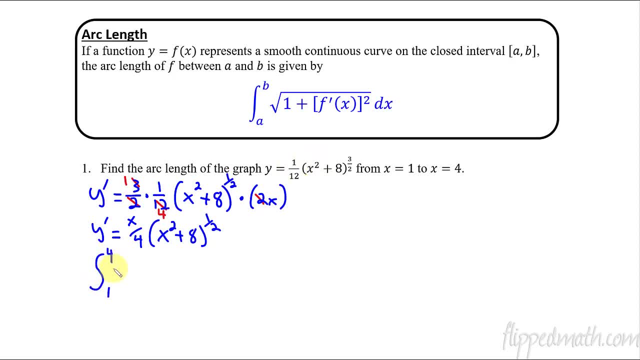 from a to B, that is, from 1 to 4, and then I'm going to say the square root of 1 plus. now I take f prime squared. so here's my f prime. so that's going to be x squared over 16. so let's go: x squared over 16. 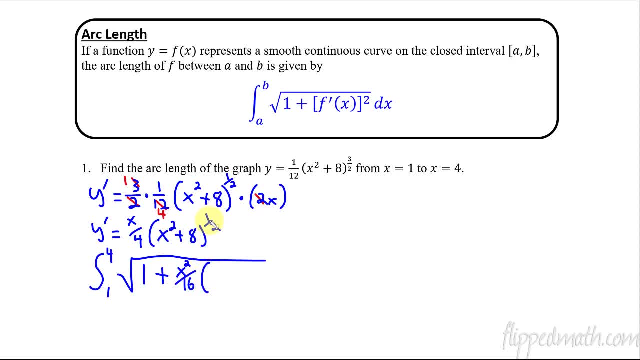 and then if I have the 1 half- and I'm squaring that- that just basically cancels out the 1 half. square root of x squared plus 8 is just x squared plus 8, so that makes that pretty simple. now it's just to the first power with respect to x. so, on the practice, you're gonna practice setting up the. 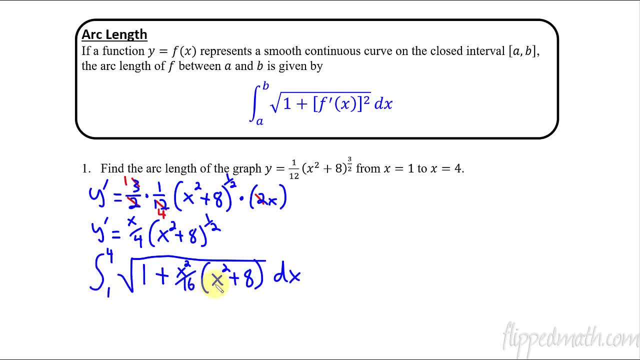 correct integral and then sometimes you'll have to solve it. I'm not gonna solve this whole thing. we've had a lot of practice with integrals and conservative integrals and I'm not gonna solve it. I'm not gonna solve this whole thing. we've had a lot of practice with integrals and integrals and 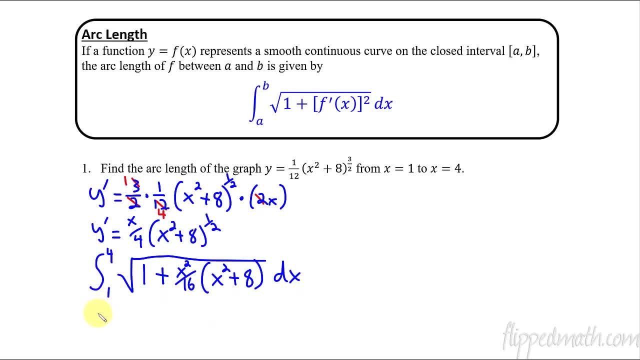 the past, since unit 6 and 7, but I do want to show you one interesting trick with this that is kind of hard algebraically to see for kids sometimes. So let me show you something I'm going to do, and that is I'm going to get rid of this. 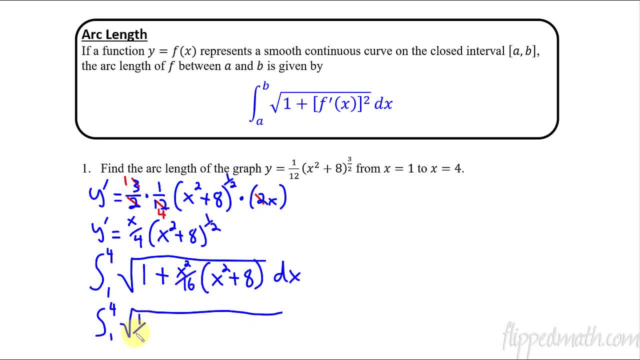 16 here by pulling out a 1 16th. So if I divide out a 1 16th to the front from this term and from this term, that 1 has to become a 16.. How do I know that? 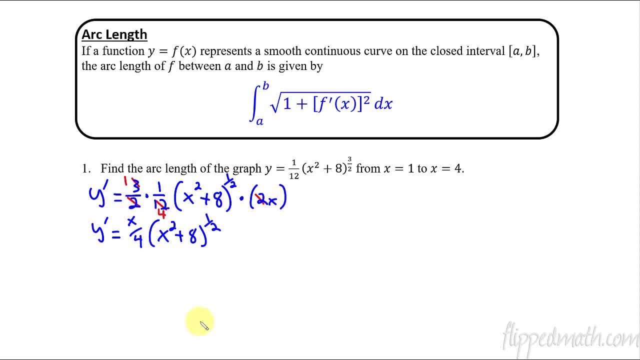 x. right there, That x is supposed to be there. so x over four. Yeah, that's important. Okay, so now I'm going to set up my integral that represents the arc length. So let's go integral from a to b, that is, from one to four, and then I'm going to say the square root of one. 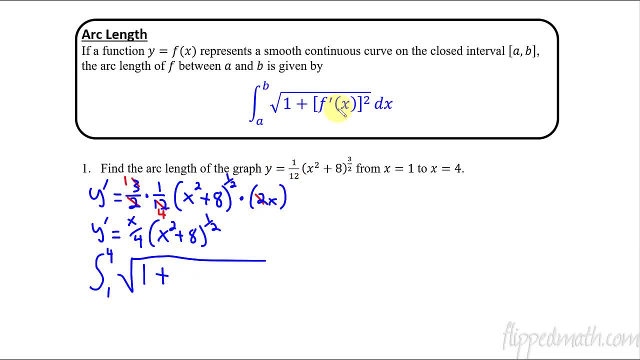 plus. now I take f prime squared. so here's my f prime. so that's going to be x squared over 16.. So let's go x squared over 16, and then, if I have the one half, and I'm squaring that. 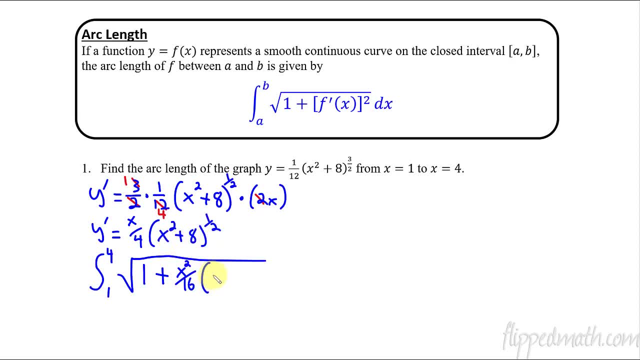 that just basically cancels out. the one half Square root of x squared plus eight is just x squared plus eight, so that makes that pretty simple. Now it's just to the first power with respect to x. So on the practice, you're going to practice setting up the correct integral. 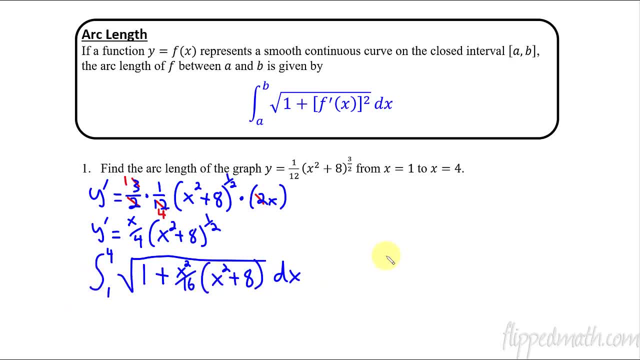 and then sometimes you'll have to solve it. I'm not going to solve it, but I'm going to solve it. I'm going to solve this whole thing. We've had a lot of practice with integrals in the past, since units six and seven, but I do want to show you one interesting trick with this. that is kind of hard. 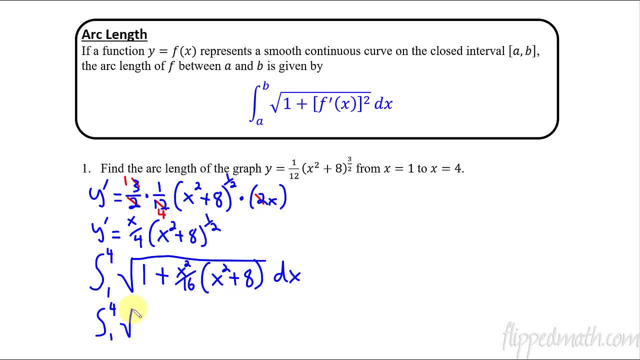 algebraically to see for kids sometimes. So let me show you something I'm going to do, and that is I'm going to get rid of this 16 here by pulling out a 1 16th. So if I divide out a 1 16th to the 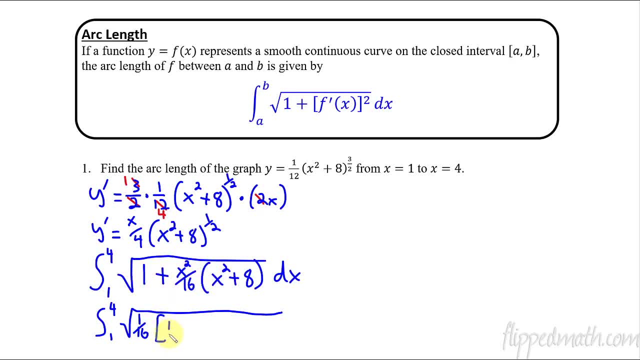 front from this term, and from this term that 1 has to become a 16.. How do I know that? Because 1 16th times 16, that'll give you my 1.. So I've just divided out a 1 16th from that plus. and now 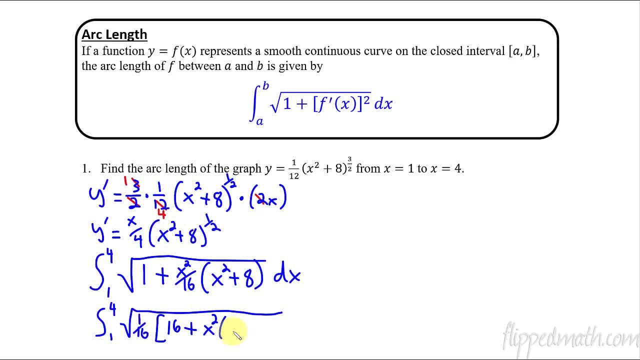 the 16 there is gone and it's just x squared, and then I have times x squared plus 8, and then close that bracket, all with respect to x. So now, what does that become? So this is now from 1 to 4,. 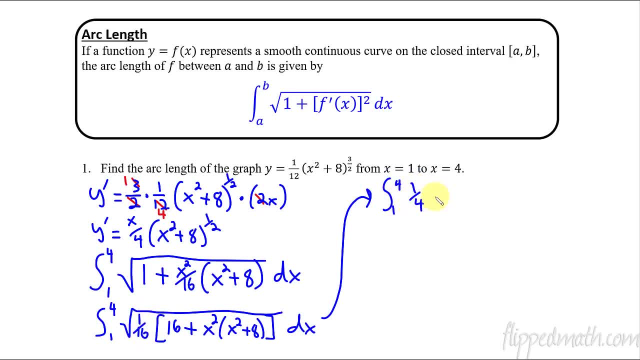 the square root of 1 16th is just 1- 4th, and then I have the square root of inside. here I have the 16 plus The x squared distributes. so I'm going to write this as x to the 4th plus 8x squared plus 16.. 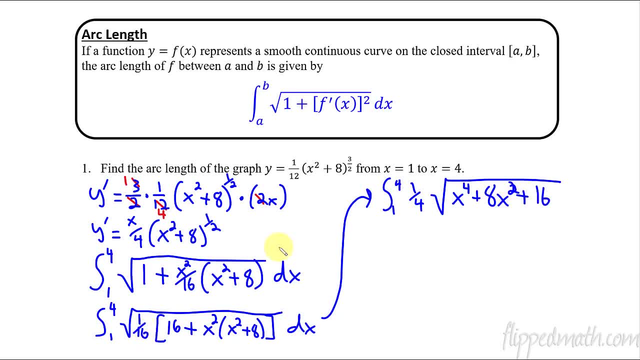 There. so that's part of the tricky part here is taking out the 1- 16th and seeing that you can reduce that, because then this would become from 1 to 4, 1- 4th. square root of that is actually a. 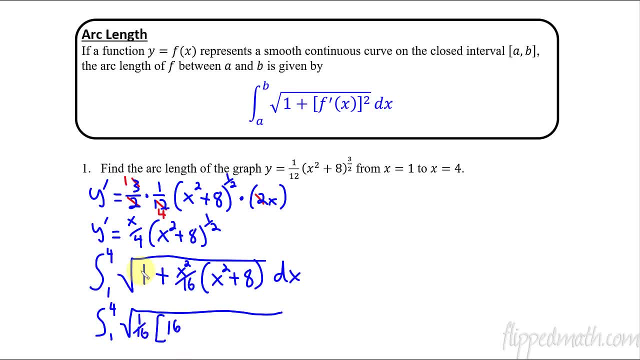 Because 1 16th times 16, that'll give you my 1.. So I've just divided out a 1 16th from that plus, and now the 16 there is gone and it's just x squared, and then I have times x squared plus 8, and then close that bracket all with. 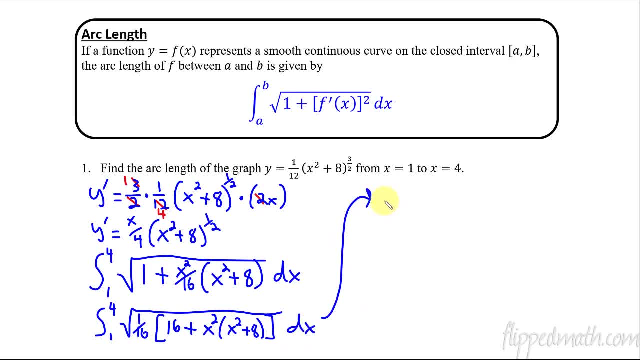 respect to x. So now, what does that become? So this is now from 1 to 4.. The square root of 1- 16th is just 1- 4th, and then I have the square root of inside. here I have the 16 plus the x squared distribute. so I'm going to write this as x to the 4th. 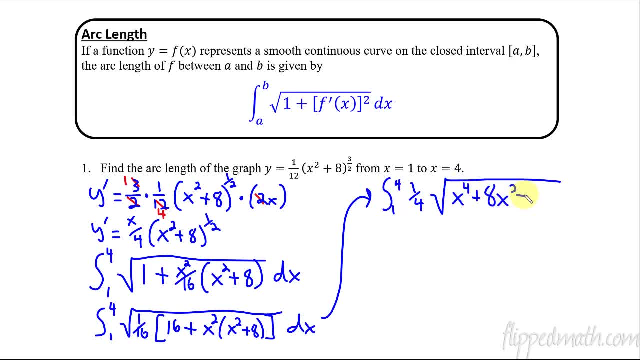 plus 1, 16th Plus 8x, squared plus 16.. There, so that's part of the tricky part here- is taking out the 1- 16th and seeing that you can reduce that, because then this would become from 1 to 4, 1- 4th square. root of that is: 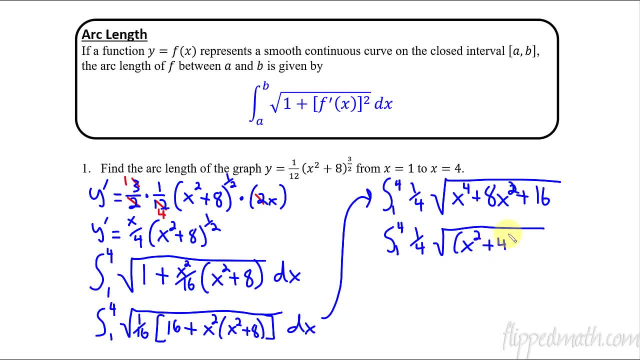 actually a perfect square of x squared plus 4, quantity squared with respect to x. Okay, so then this square root and the squared would cancel and you could work from here. So this is 1, 16th times x squared plus 4 with respect to x, and then, if you work through that whole thing- I'm not going to work through that, but if you work through that whole thing- the answer would be 33 4ths once you finish it all up. 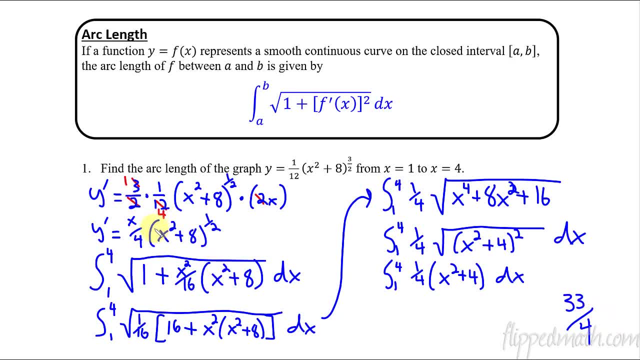 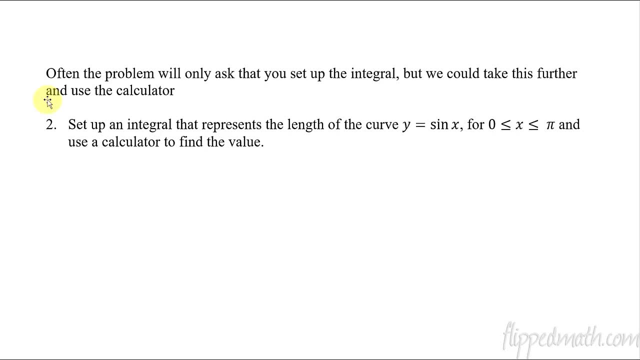 Okay. so again, that was just to show you the setup, how you set this formula up. but then there is sometimes some challenging little ways to manipulate the integral into something that you can work with. All right, let's just do one more example here, and then I'll show you the proof, and that is for this one. we're going to use a calculator, so this one's nice and easy. 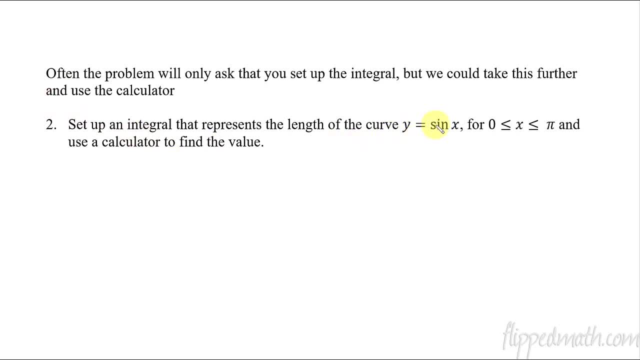 Let's just set up real quick. How do we do this? So, if we have the curve, y equals sine x. so we got a sine curve over and over and over again with a wave curve, and we're just figuring out first the derivative right. because what is it again? 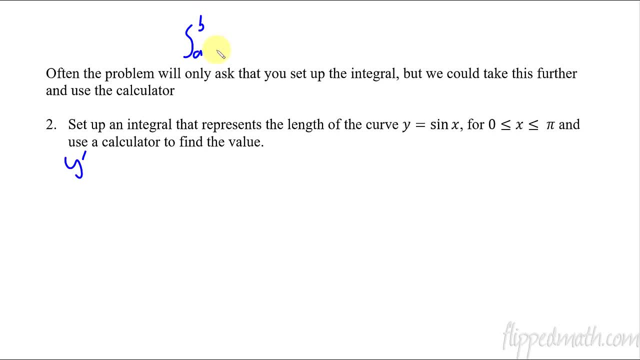 It's from a to b and then it is a square root of 1 plus f prime, but then it's squared with respect to x, So y prime equals. we've got to figure out that derivative. that's pretty simple, it's just cosine x and then, if we square that, 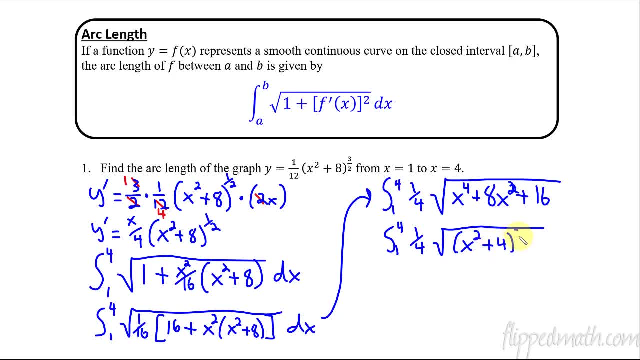 perfect square of x squared plus 4, quantity squared with respect to x. Okay, so then this square root and the squared would be 1- 4th. So I'm going to write this as x to the 4th plus 8x squared. 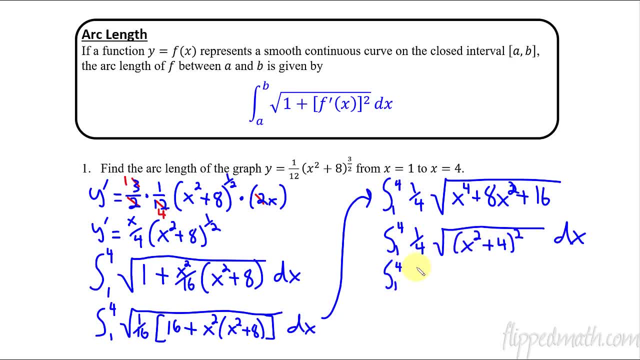 cancel and you could work from here: 1 4th times x squared plus 4 with respect to x, and then, if you work through that whole thing- I'm not going to work through that, but if you work through that whole thing- the answer would be 33 4ths once you finish it all up. Okay, so again, that was just to. 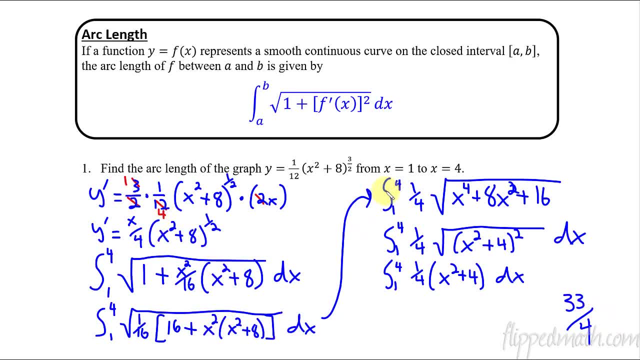 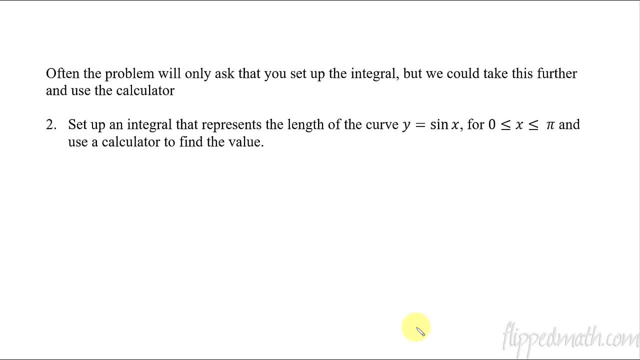 show you the setup, how you set this formula up. but then there is sometimes some challenging little ways to manipulate the integral into something that you can work with. All right, let's just do one more example here and then I'll show you the proof, and that is for this one. we're 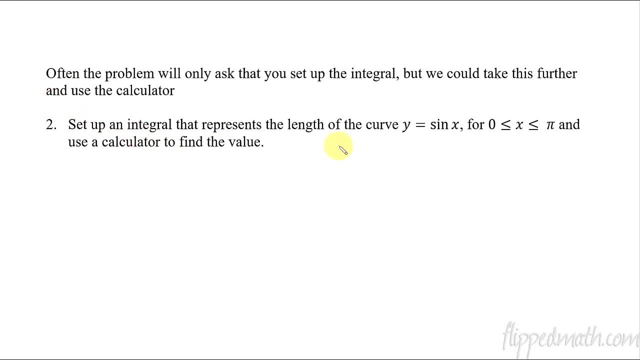 going to use a calculator, so this one's nice and easy. Let's just set up real quick. how do we do this? So, if we have the curve, y equals sine x. so we got a sine curve over and over and over again with a wave curve, and we're just figuring out first the derivative right. because what is it? 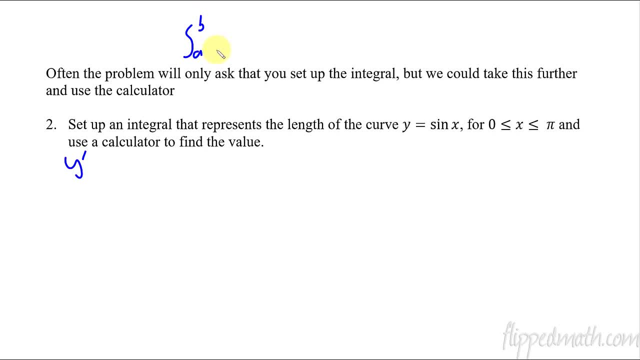 again, It's from a to b and then it is a square root of 1 plus f prime, but then it's squared with respect to x, So y prime equals. we've got to figure out that derivative. that's pretty simple. 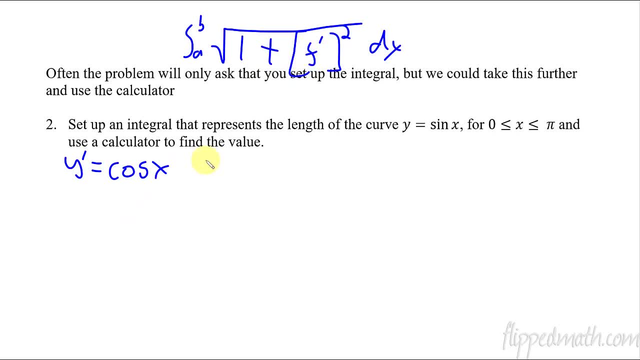 it's just cosine x, and then if we square that we would just get: so y prime squared would just equal cosine squared x. All right, so we have from a to b, so a is a 0, and then b is pi, and then we 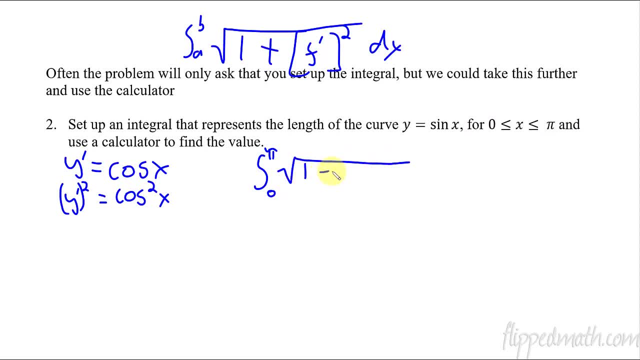 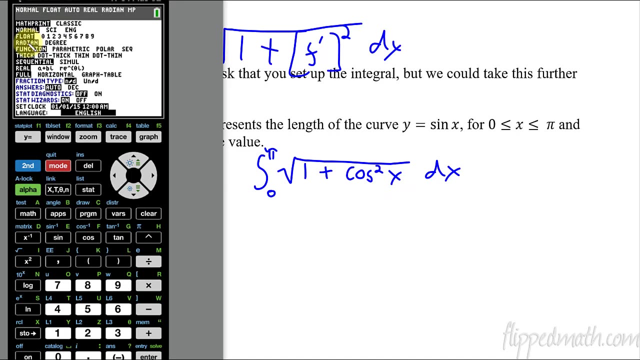 say the square root of 1 plus cosine squared x with respect to x. and now let's use our calculator. So I'm going to pull up my calculator. I'm typing in a cosine value, so let's just double check that the mode is in radians. yes, it is. 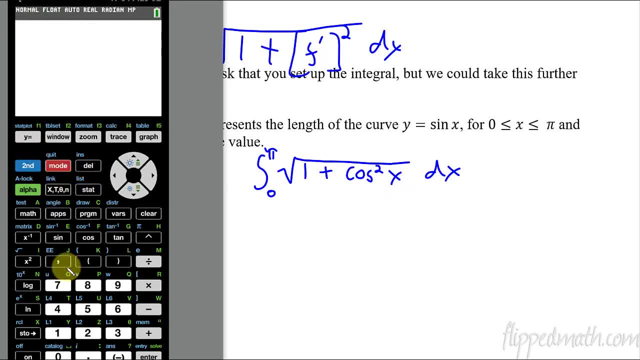 so I'm good there. So, whoops, get out of this. So then we go, math 9, math option 9, from 0 to pi, and then the square root of 1 plus cosine squared, And so the way you do, cosine squared again. 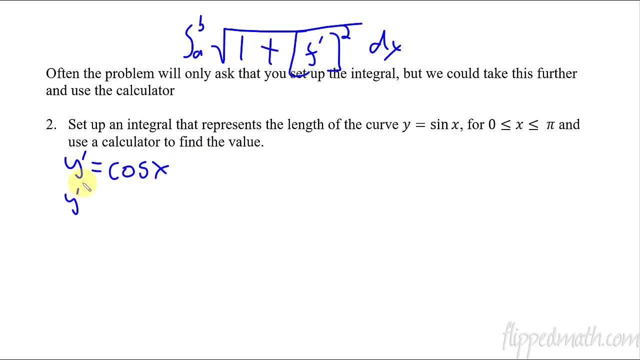 we would just get so y prime squared would just equal cosine squared x. All right, so we have from a to b, so a is a zero and then b is pi, and then we say the square root of 1 plus cosine squared x with respect to x. 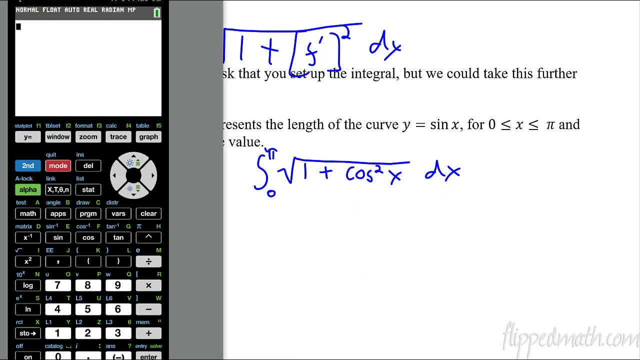 And now let's use our calculator. so I'm going to pull up my calculator. I'm typing in a cosine value, so let's just double check that the mode Is in radians. yes, it is, so I'm good there. So, whoops, get out of this. 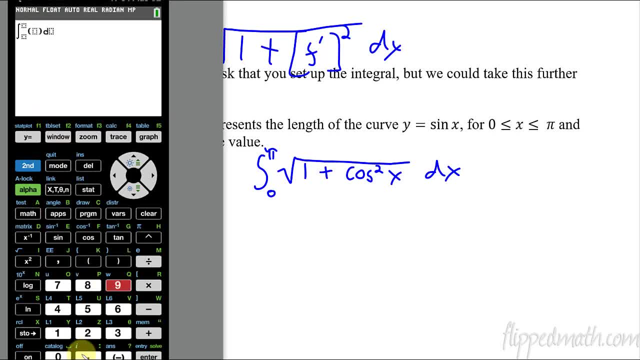 So then we go math 9, math option 9, from 0 to pi, and then the square root of 1 plus cosine squared, And so the way you do, cosine squared, again it's cosine x, close the parenthesis and then square it. 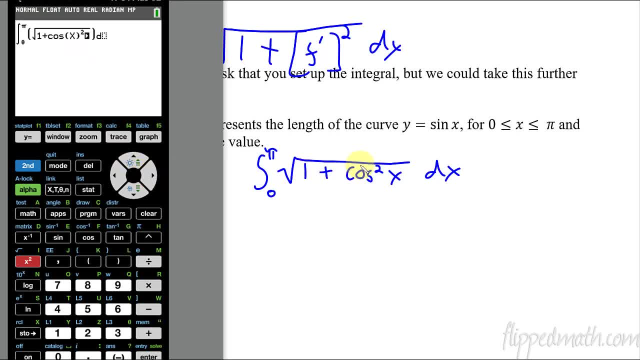 That's not x squared right there, that is actually cosine x squared. so cosine squared x is what that looks like. And then with respect to x. so what is the answer to that one? 3.820.. 3.820, truncated and rounded is the same, so 3.82.. 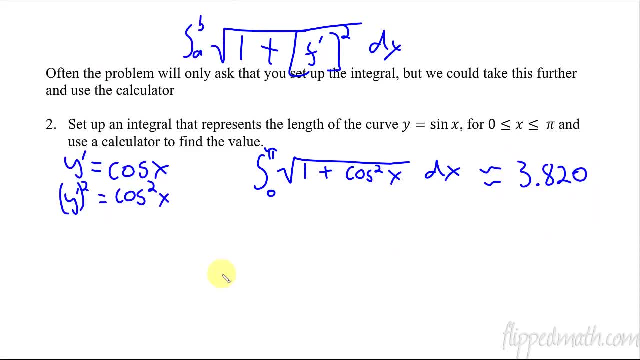 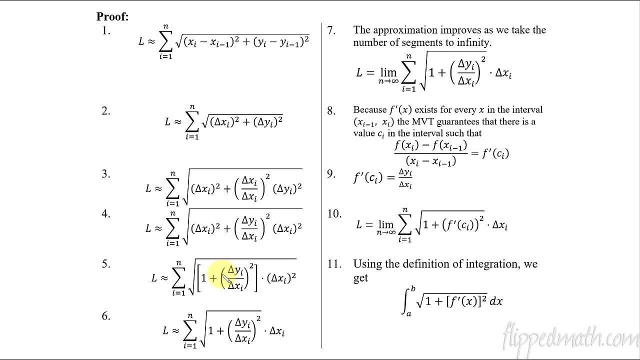 I'll go ahead and tag on the zero there at the end, but that is the answer. Okay, so that's everything in this lesson. that's it All I'm going to do now. so those of you who aren't mathematically inclined and don't want to learn something really cool from the proof, I guess you are done. 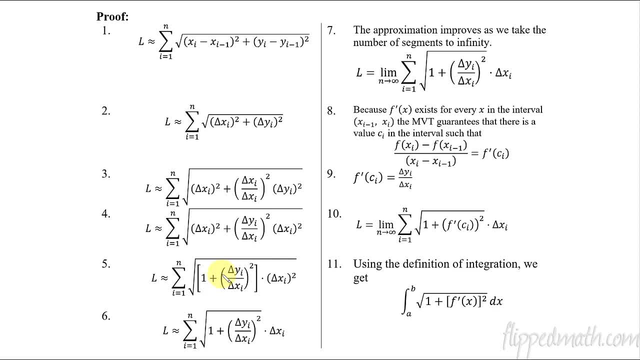 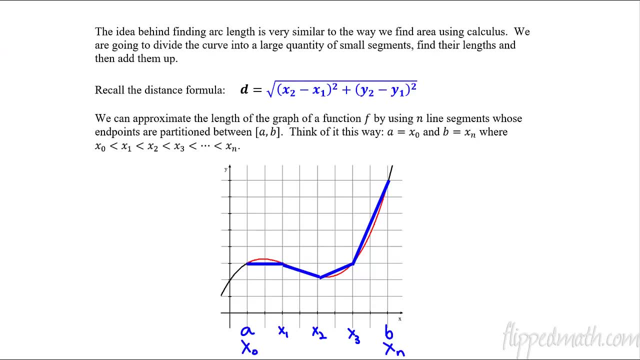 This proof. let me just show this to you real quick. This is not that bad and I've left it on your notes so you didn't even have to write all of this out. Let me just explain it to you real quick, and it goes all the way back to what we did on this part of your notes here. 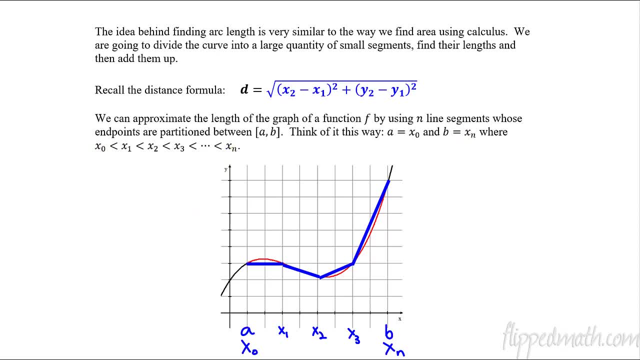 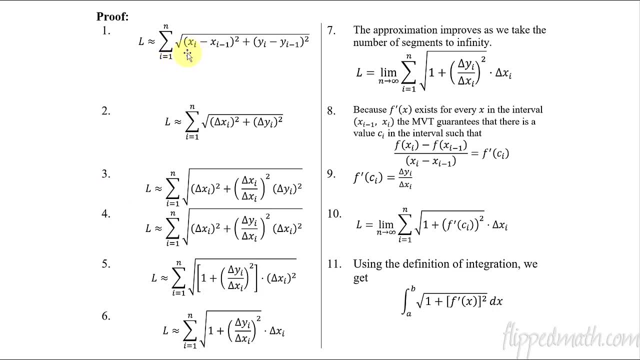 Where we said from x0. To x to the nth. So you can see here x to the i. What does this mean? So i is just any particular segment. So if it's a 1, it's the first segment. 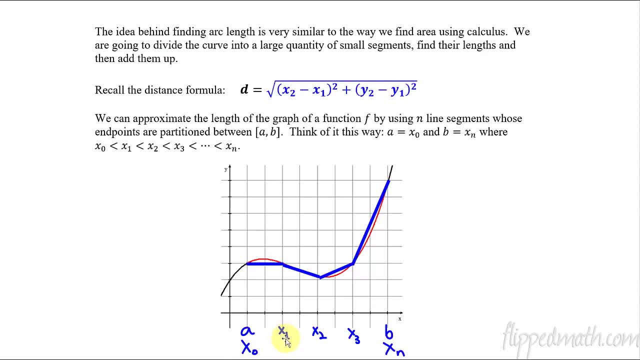 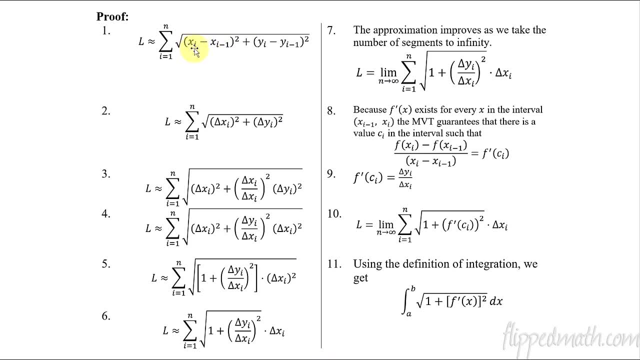 If it's a 2, it's the second segment. Let me show you that. So if this is x1, that's the first segment. x2, it's talking about the end of the second segment. So if we do x3 minus x to the 2, because it would be 3 minus 1, so it's the difference for that segment. 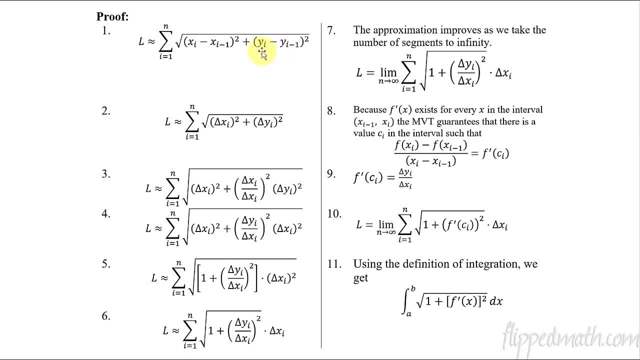 So it's the difference of x's the difference of y's, so it's just the distance formula. What we're doing is we're summing up all of those. we're summing them all up, from 1 to n, however many little segments we have. 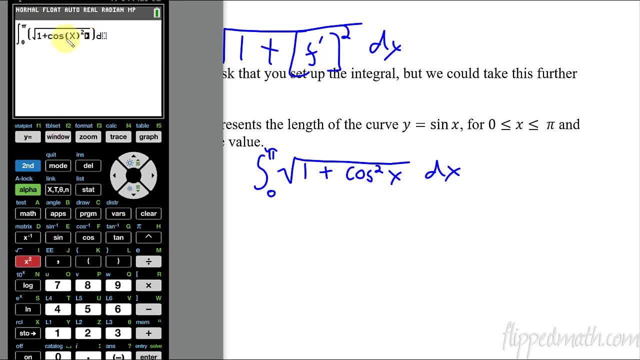 it's cosine x. close the parenthesis and then square it. That's not x squared right there, that is actually cosine x squared. so cosine squared x is what that looks like. And then the square root of x. so what is the answer to that one? 3.820, truncated and rounded is the same. 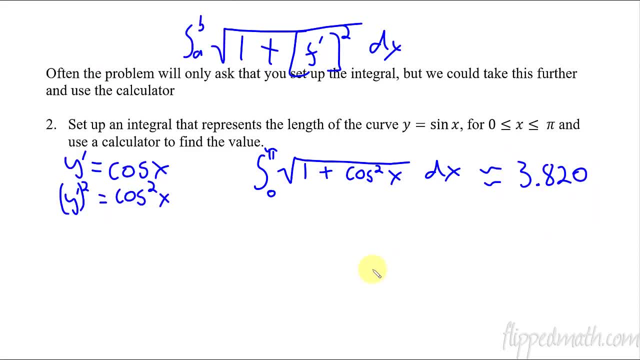 so 3.82.. I'll go ahead and tag on the 0 there at the end, but that is the answer. Okay, so that's everything in this lesson. that's it All I'm going to do now. so those of you who aren't. 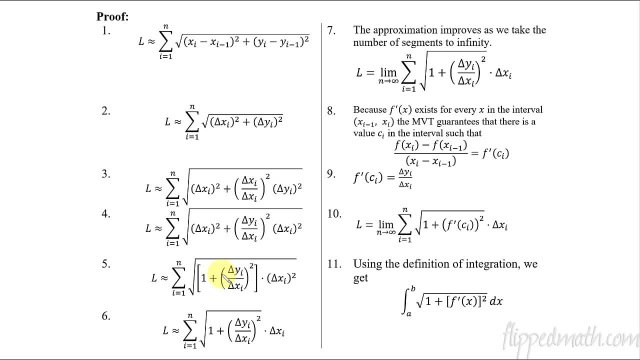 mathematically inclined and don't want to learn something really cool from the proof. I guess you are done This proof. let me just show this to you real quick. This is not that bad and I've left it on your note so you didn't even have to write all of this out. I just let me just explain it to you. 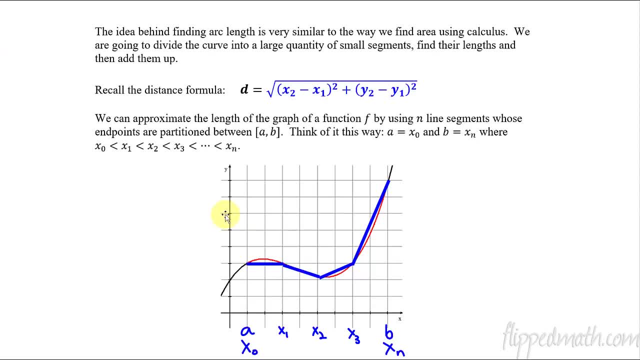 real quick and it goes all the way back to what we did in the last lesson. So let's go back to the on this part of your notes here where we said from x0 to x to the nth. So you can see here. 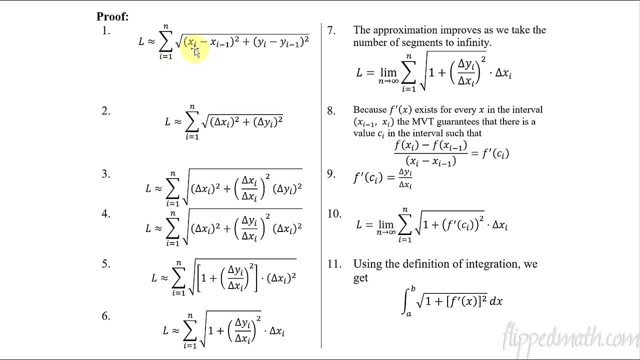 x to the i. What does this mean? So i is just any particular segment. So if it's a 1, it's the first segment. If it's a 2, it's the second segment. Let me show you that. So if this is x1,. 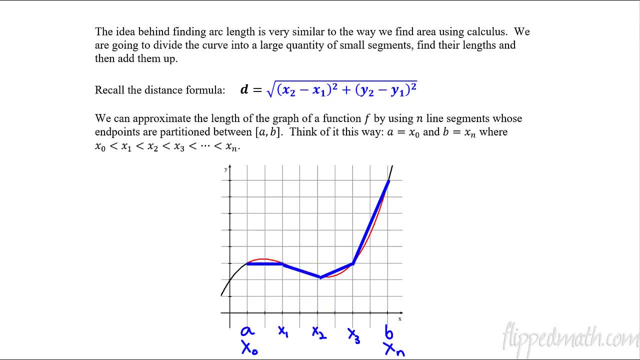 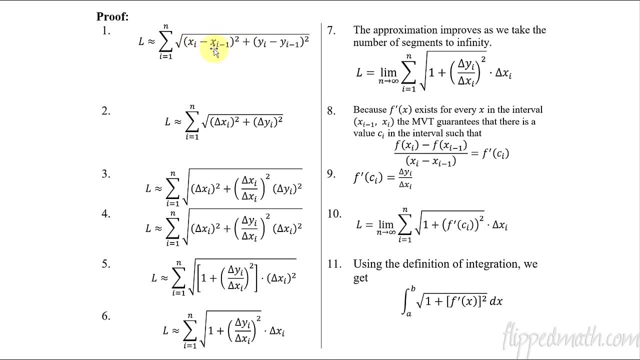 that's the first segment. x2, it's talking about the end of the second segment. So if we do x3 minus x to the 2, because it'd be 3 minus 1. So it's the difference for that segment. So the difference of x's. 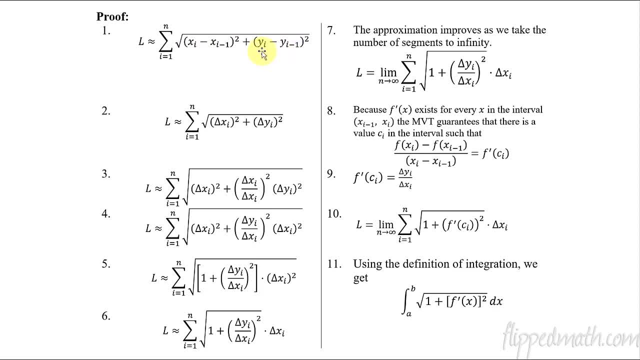 difference of y's. So it's just the distance formula. What we're doing is we're summing up all of those. We're summing them all up, from 1 to n, however many little segments we have. Well, that's just this: The difference in x's, the difference in y's. So now, what did I do from? 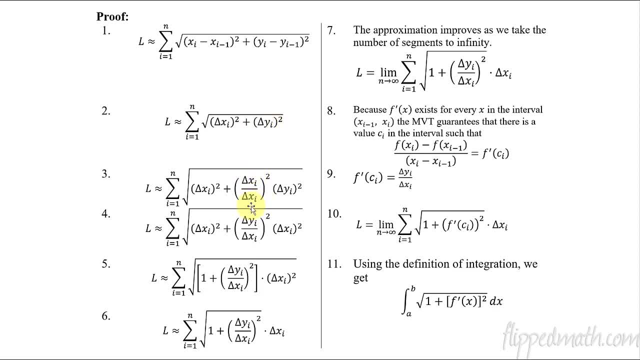 this step to this step. I tagged on a delta x over delta x. Okay, that's just 1 squared. Okay, that's fine, You can do that 1 squared. And then you can see: here I swapped the delta y and the delta x's, It's just doing a. 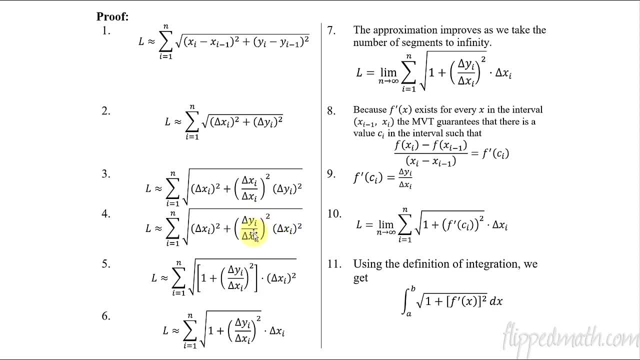 little bit of some manipulation here with the numbers, So that becomes this. So now I factored out a delta x squared. See this: There's a delta x- i, delta x sub i squared. If you factor them out, it becomes 1 plus this. Okay, So now what does that become? The square root of delta x, little i. 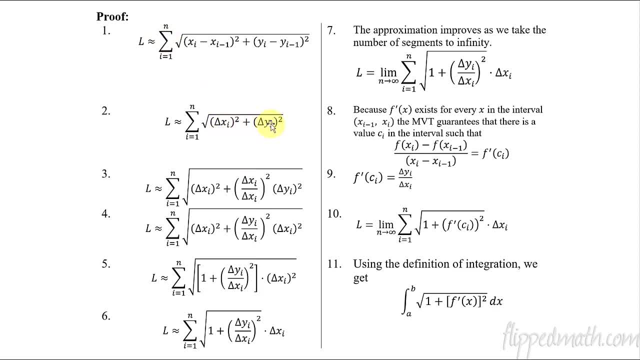 Well, that's just this: the difference in x's, the difference in y's. So now, what did I do? from this step to this step, I tagged on a delta x over delta x. Okay, that's just 1 squared. Okay, that's fine, you can do that. 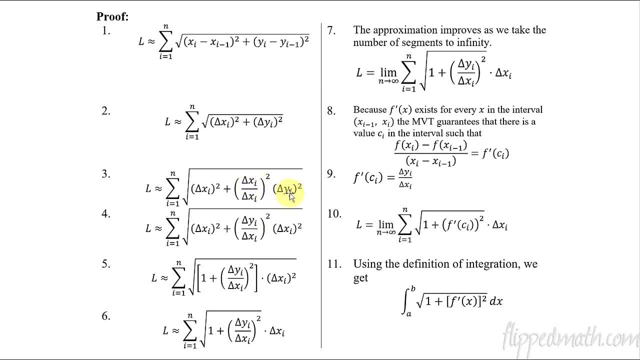 1 squared. And then you can see here I swapped the delta y and the delta y And the delta x's. it's just doing a little bit of some manipulation here with the numbers, So that becomes this. So now I factored out a delta x squared. 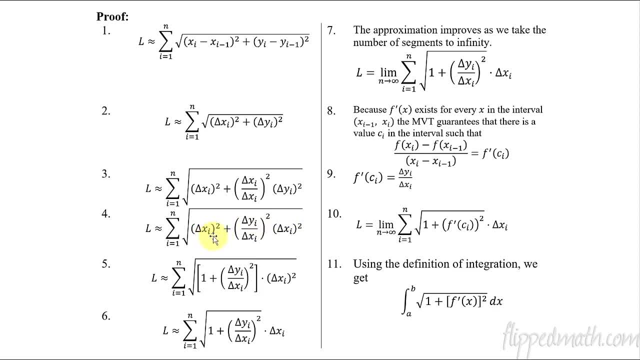 See this: There's a delta x i, delta x sub i squared. If you factor them out, it becomes 1 plus this. Okay, so now what does that become? The square root of delta x? little i squared is just delta x i. 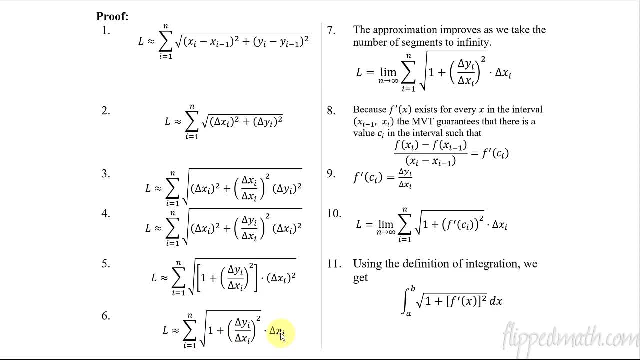 So now we're down to this one. This is confusing, I know. Trust me, it took me forever to make sure I understood this all. And I'm just doing this real fast because, again, on the AP exam, you won't have to manipulate this at all through this proof. 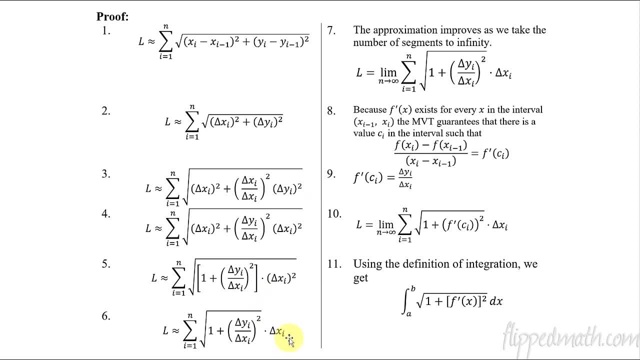 But it is nice to know where this arc length comes from. It's kind of a nice little activity on the side, if you wanted to understand it. And then what do we have here? Approximation. Approximation improves as we take the number of segments to infinity. 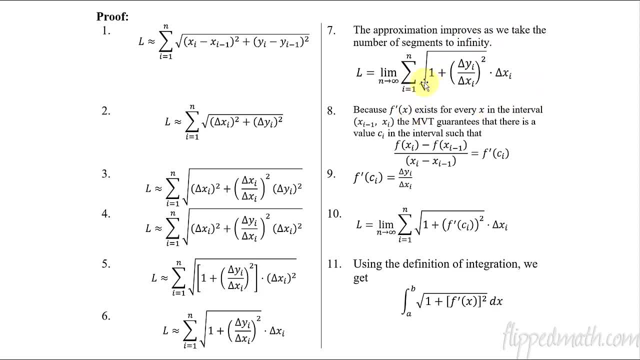 So if we say just this summation notation here, if we say that n is going to approach infinity, that means we're going to end up with the arc length. So we take this same summation and say it approaches infinity. So here's the crazy thing. 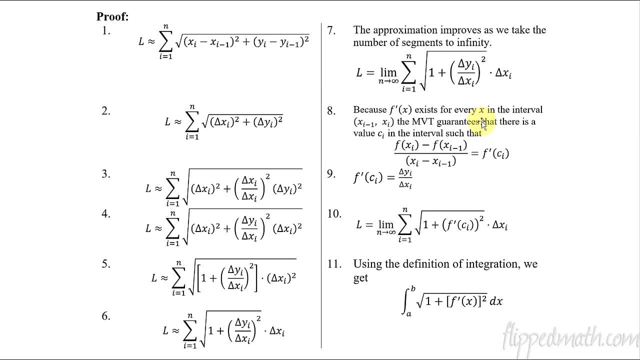 So this is using the mean value theorem. Since we can take any one of those little segments, we can use the mean value theorem for any one of the segments and say that there's some c inside that segment where the derivative equals the average. Okay, so now what this can lead us to is this: f of x i minus f of x- i minus 1.. 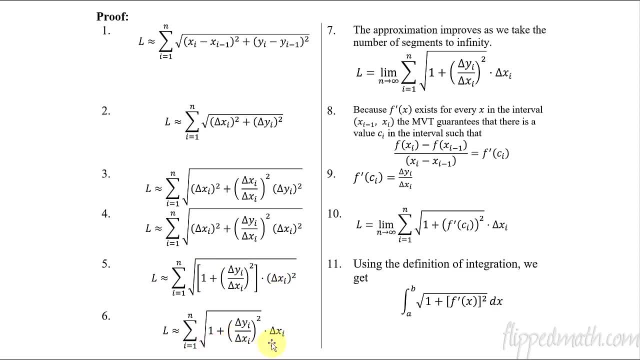 squared is just delta x, i. So now we're down to this one. Yeah, this is confusing, I know. Trust me, It took me forever to make sure I understood this all. And I'm just doing this real fast because again, on the AP exam, you won't have to manipulate this at all through this proof. 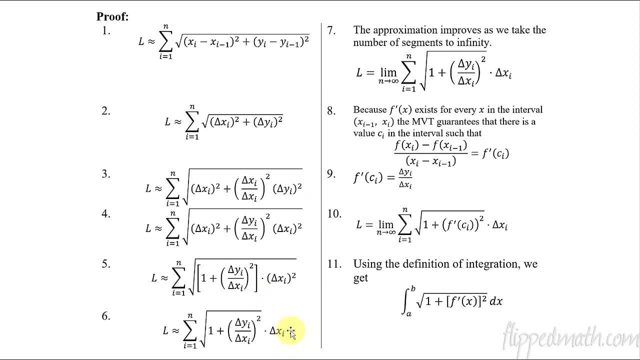 but it is nice to know where this arc length comes from. It's kind of a nice little activity on the side, if you wanted to understand it. And then what do we have here? Approximation. Approximation improves as we take the number of segments to infinity. So if we say just this: 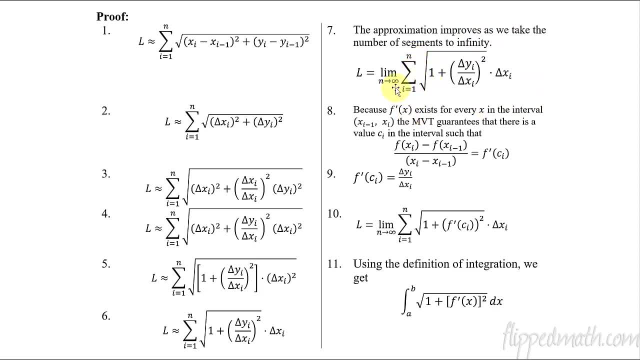 summation notation here. if we say that n is going to approach infinity, we're going to have an infinity. That means we're going to end up with the arc length. So we take this same summation and say it approaches infinity. So here's the crazy thing. So this is using the mean value. 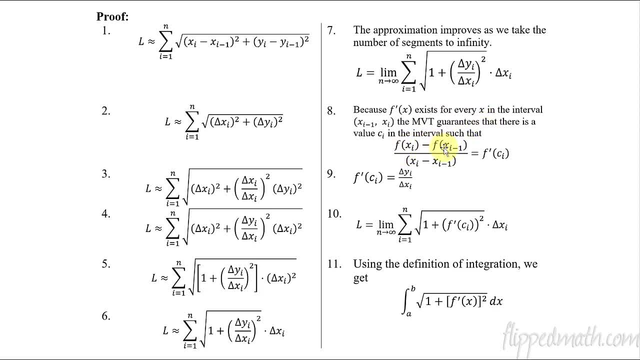 theorem. Since we can take any one of those little segments, we could use the mean value theorem for any one of the segments and say that there's some c inside that segment where the derivative equals the average. Okay, So now what this can lead us to is this: 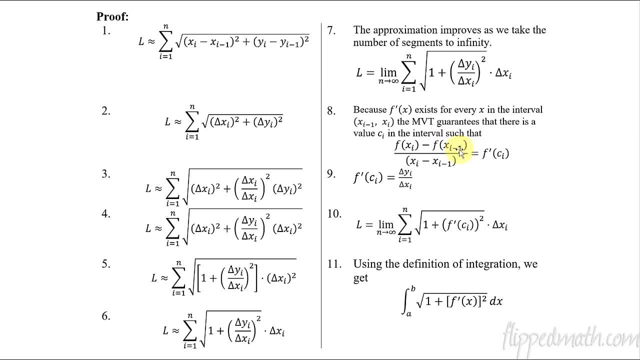 f of xi minus f of xi minus 1.. That's basically delta y over delta x. Okay, So let's go back here This delta y over delta x, that was right here. Delta y over delta x, that is equivalent. 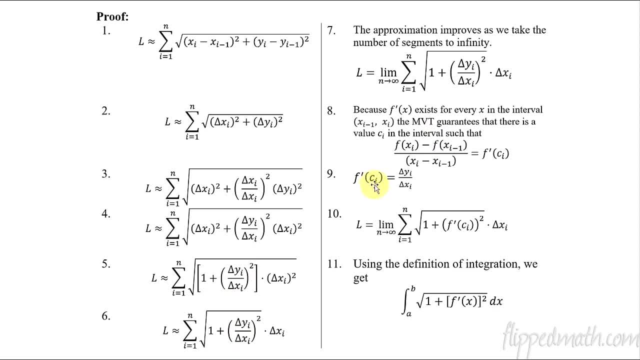 to saying f prime of some c with the mean value theorem. So now we just replace that there with f prime of c. And then this leads us to back in unit 6, we did integration like the definition of an integral and how we worked with summation notation, And then we did integration like the. 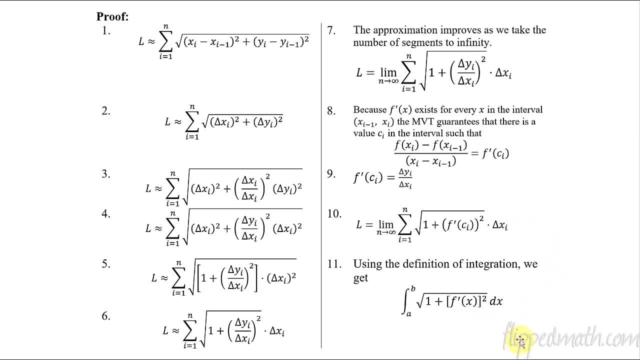 definition of an integral and how we worked with summation notation, And it leads us to this Holy cow that is confusing. So that's the proof of how we come up with this arc length stuff. Again, don't stress about this, You don't have to know that, You really just need to know this part. 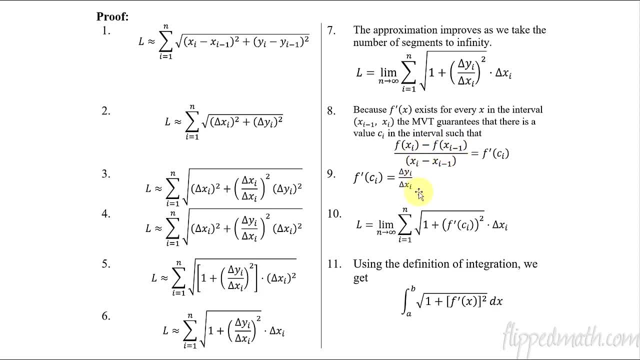 That's basically delta y over delta x. Okay, so let's go back here This delta y over delta x, that was right here. Delta y over delta x, that is equivalent to saying f prime of some c with the mean value theorem. 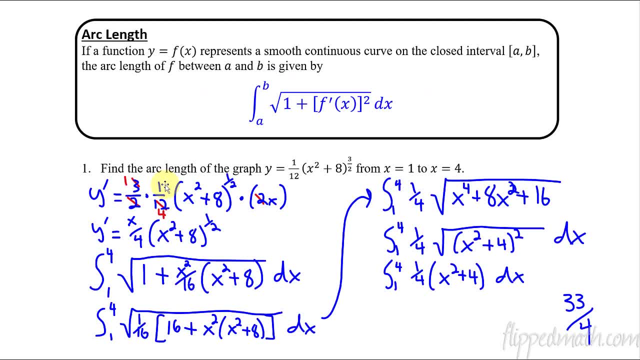 right here how to use the formula and how to plug it in. Just don't forget that it's f prime, not f squared. It's f prime squared. Okay, That's everything, Mr Bean, signing off here. Rock that, master check, And I will see you back in our next unit, which is just for the BC students. Bye-bye.